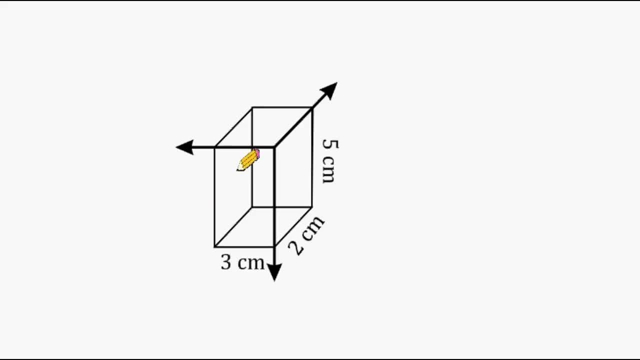 of the rectangular prism. So we could say that this is the length, the width and the height, And you can really do that with any corner of the rectangular prism. If we were to select this corner, we could look at these three lines as representing the three dimensions. 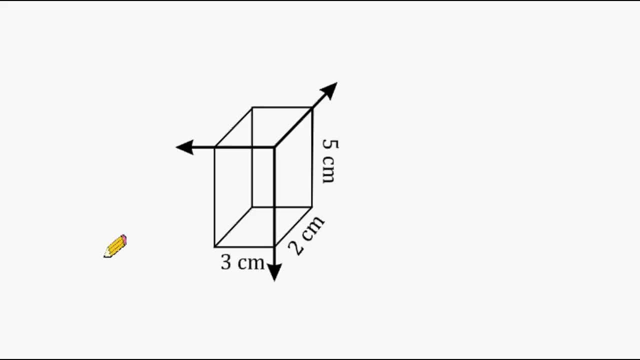 of the rectangular prism. Now if you look at this corner and the three lines that emanate from that single point, we should notice that it kind of forms a Y figure. So what we're going to do is take that Y figure and use it to calculate the 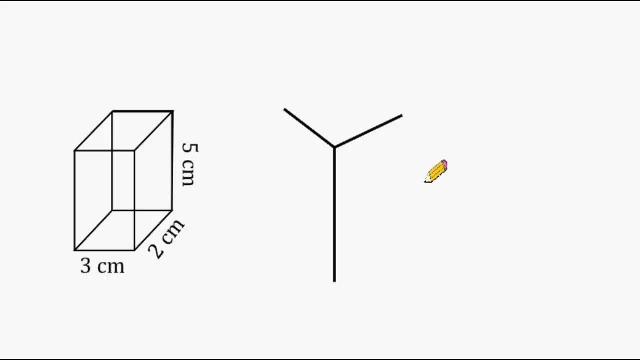 surface area of our rectangular prism. So when calculating the surface area of any rectangular prism, the first thing that you can do is draw what looks kind of like a letter Y, and each one of these lines represents each one of the three dimensions of the rectangular prism: The length, the width and the height. So 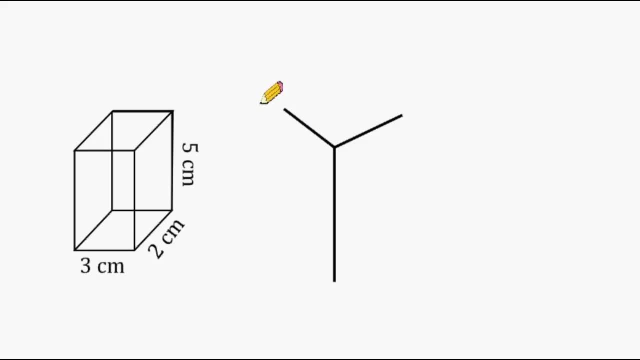 let's take our shortest line and write our smallest number, which is a number two. Then we're going to put a number three here and a number five here, And it really doesn't matter which order you write these numbers. you will end up getting the same answer anyway. 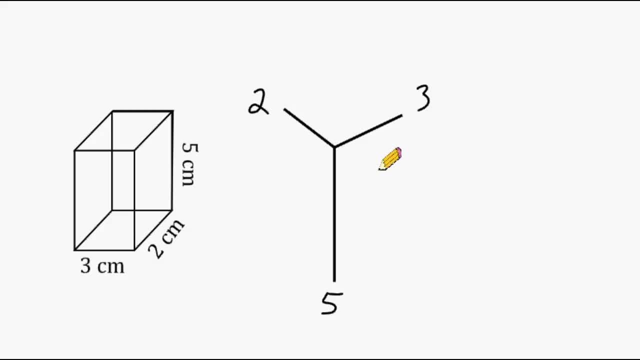 Now what we have to do is just select two numbers at a time and multiply them. So let's start with the two and the three. Two times three is six, and what we're going to do is write that answer where these two lines converge on each other. 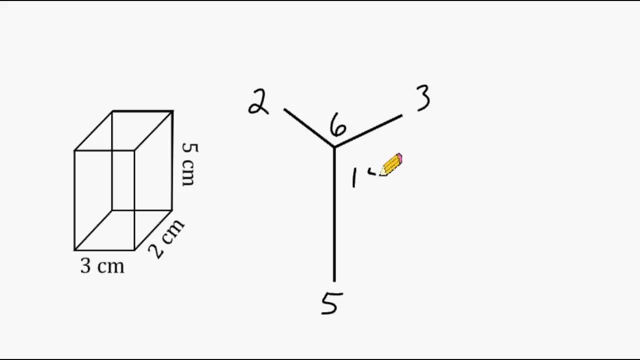 Next, let's do three times five, which is fifteen, and two times five is ten. Now what these three numbers represent are the areas of the front, three surfaces. But remember for each surface there is an equal or congruent surface. For example, this top surface would be: 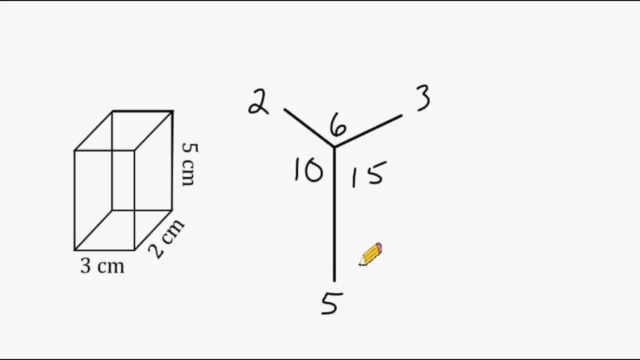 six square units, which means the bottom surface would also be six square units, And we would have two rectangles with an area of fifteen and two rectangles with an area of ten square units. So what we do after getting these three numbers is we take those and we add them together.